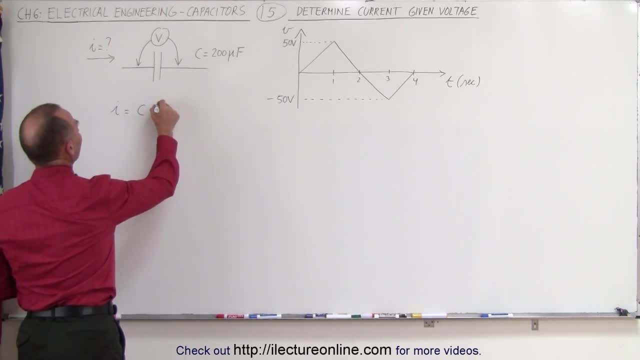 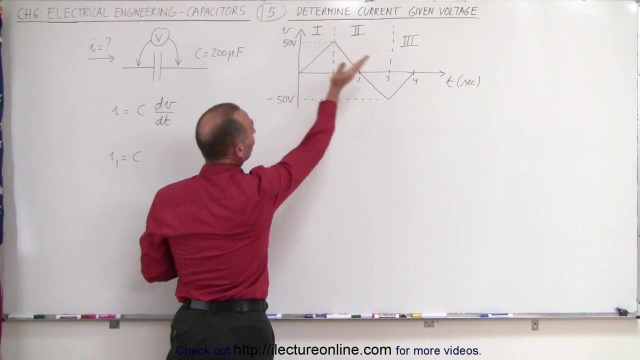 follows: I is equal to the capacitance times the change in the voltage with respect to time. That means that the current in region 1 is equal to the capacitance times the change in voltage over time. In other words, that's equal to the slope of this voltage versus time graph. So that's 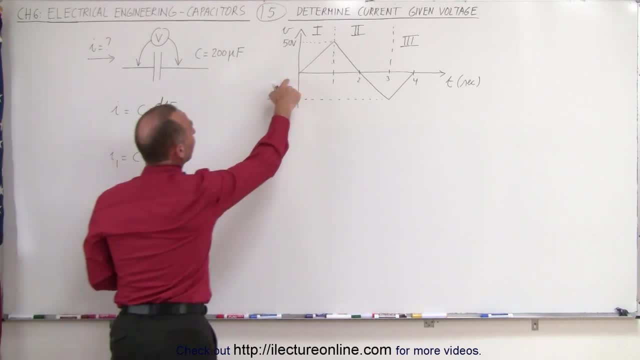 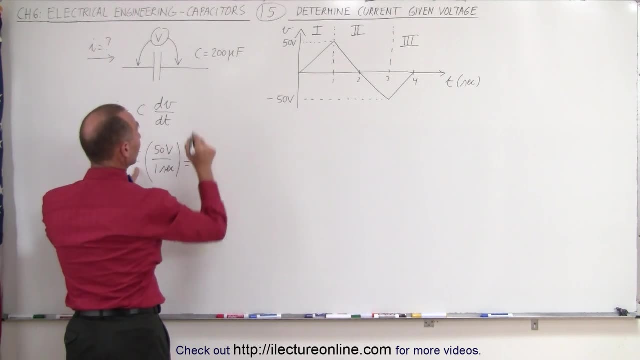 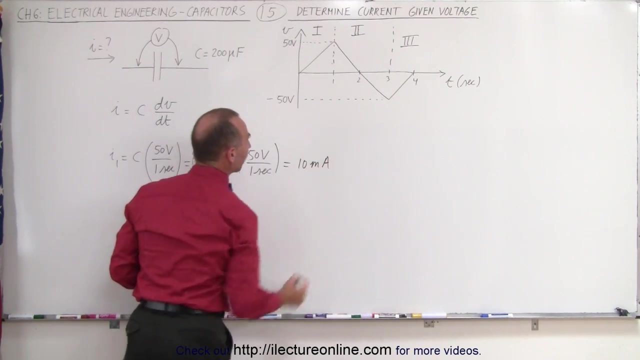 equal to dvd, And the change in the voltage over time is a change of 50 volts divided by 1 second. And since the capacitance is 200 microfarads, we write 200 microfarads times the ratio of 50 volts divided by 1 second, which means we have a current of 10 milliamps. 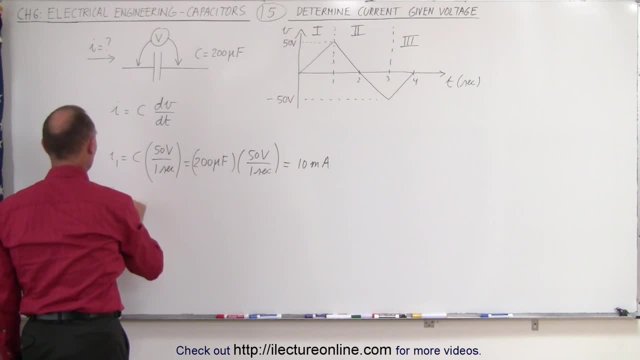 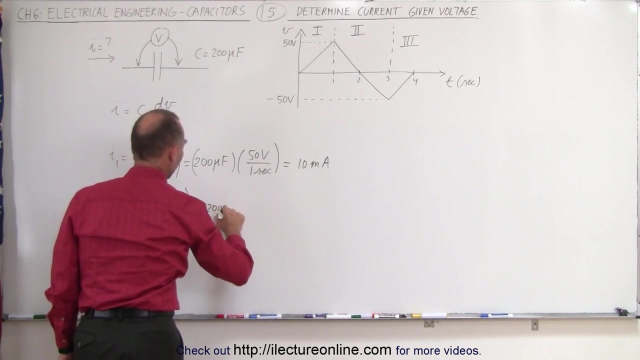 Then we do this again for the second region. So the current in the second region is equal to the capacitance times the change in the voltage over time. so it's minus. the total change in the voltage is 100 volts over a period of two seconds and since the capacitance is 200 microfarads. 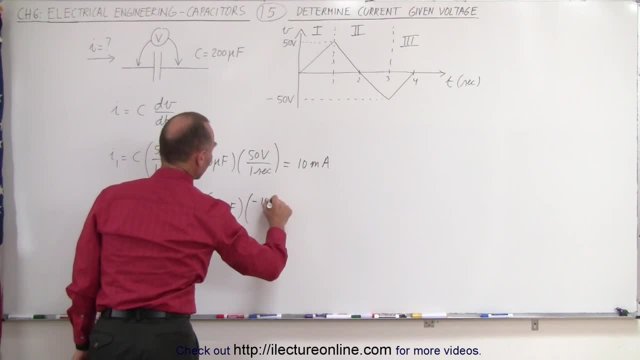 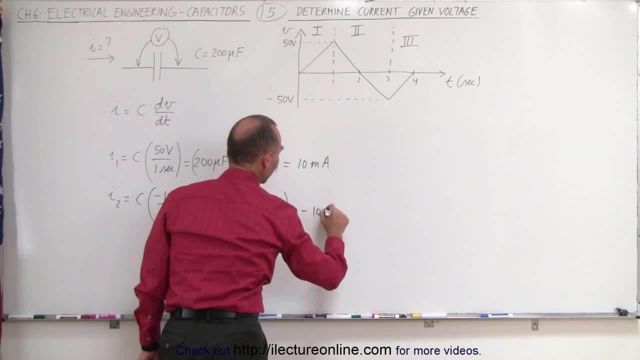 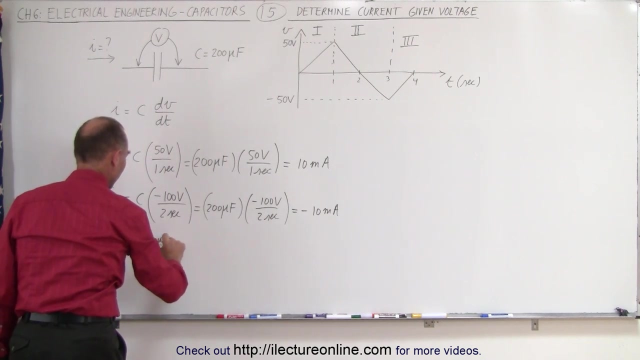 multiplying that times minus 100 volts over two seconds and looks like the magnitude is the same with a different sign. so this is minus 10 milliamps. and then again for region 3: I3 is equal to the capacitance, which is 200 microfarads times the rate of change of the voltage over time, which 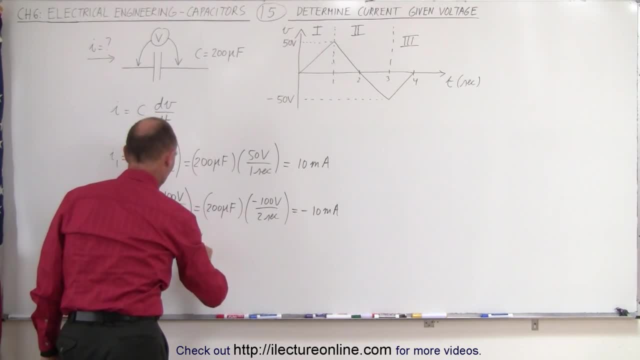 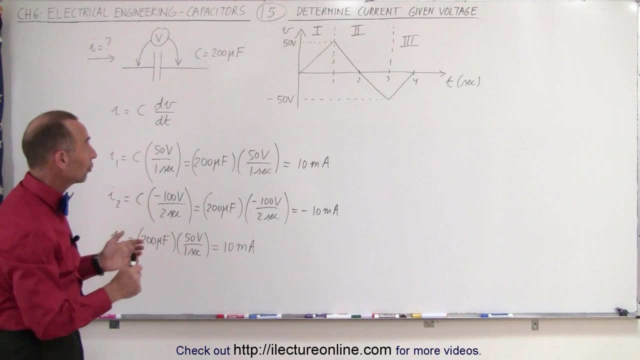 is 50 volts over one second. 50 volts over one second, which is again 10 milliamps. so that's how we determine the current through a capacitor. when there's no resistor involved, it's simply determined by the equation: i equals c, dv, dt determine the change of the voltage over time. 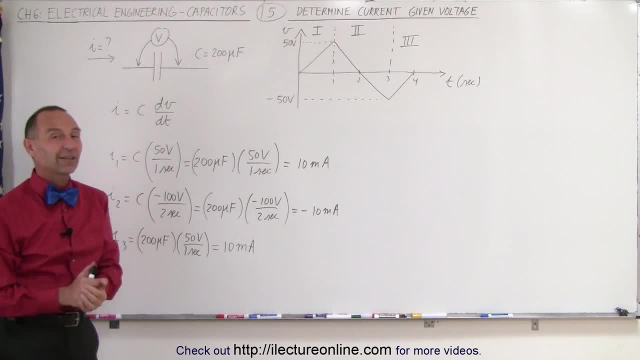 and you get the current. if you know the capacitance you and that's how it's done.